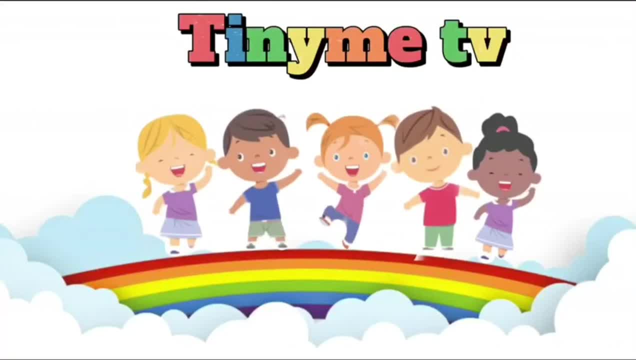 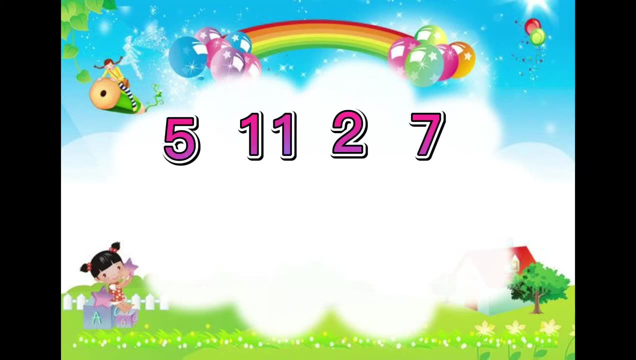 Welcome to TinyMeTV. Today we are arranging numbers from least to greatest. Can you identify these numbers? 5, 11, 2, 7. Let's arrange these numbers from least to greatest: 2, 5, 7, 11. Let's try another one. 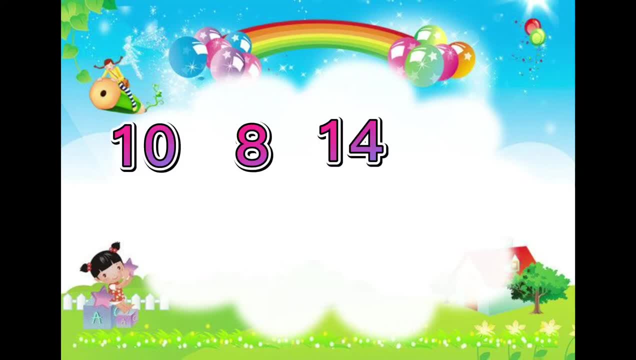 10, 8, 14, 2. Let's arrange these numbers from least to greatest. Which number from this set is the smallest? Did I hear 2?? Yes, great job. The smallest number here is 2.. Next in line is the number 8.. 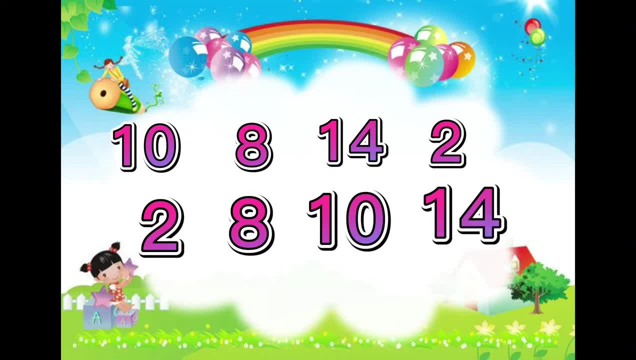 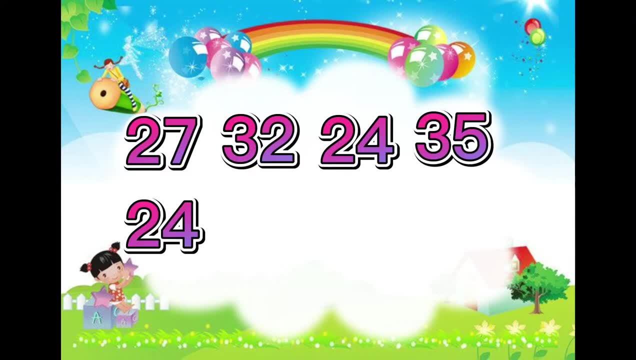 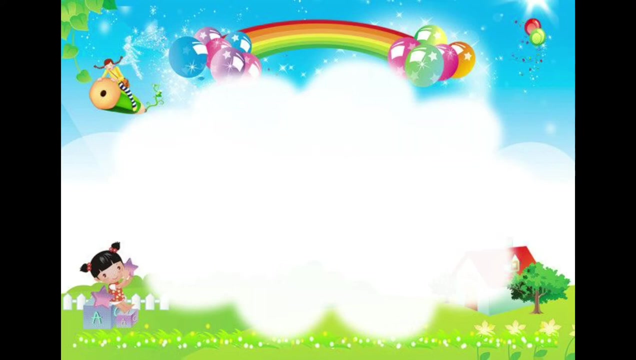 After that is the number 10.. Lastly is the number 14.. Let's try some more. The smallest number in this set is 24.. Afterwards is 27., Then 32. And lastly 35. You're doing awesome so far. 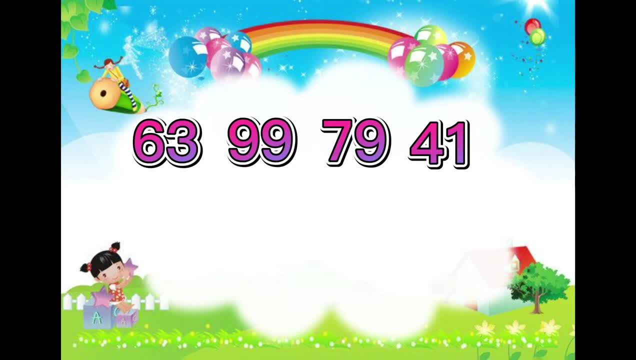 Here's another set of numbers we're going to arrange. Can you guess? the smallest number Is the smallest number of the set, 41?. Yes, Great job, Jayden. What's next? Yes, 63.. 79.. And lastly, 99.. 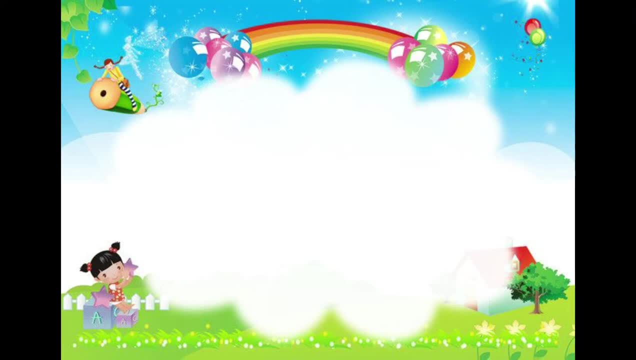 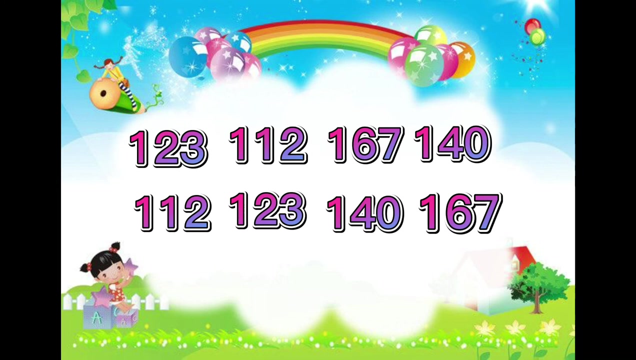 Here is the last set of numbers: 100.. 123. 112. 167. 140.. The smallest number in this set is 112.. After that is 123.. 140 is the next number in line And the final number is 167.. 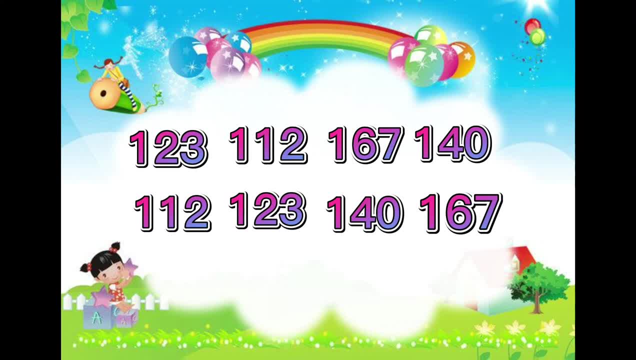 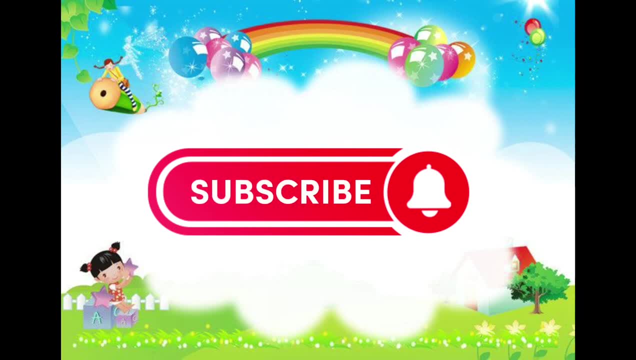 Now you know how to arrange numbers from least to greatest. Thanks for tuning in with TinyMeTV. Subscribe to my channel for more videos. See you next time. Bye.